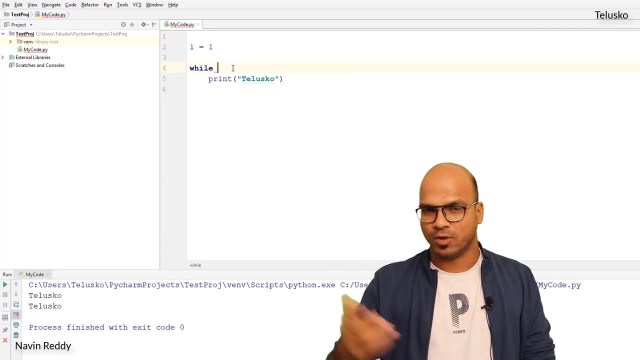 will say: I starts with one, and then every time. Okay, first of all, you have to check, right. How will I check if the value of I is less than equal to five? Okay, we have to apply a condition, right? So step one would be: take a counter, a variable. 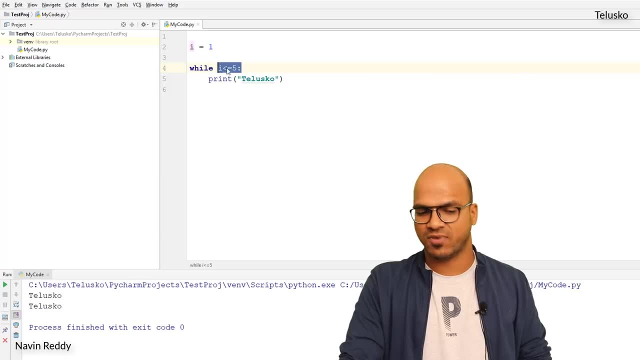 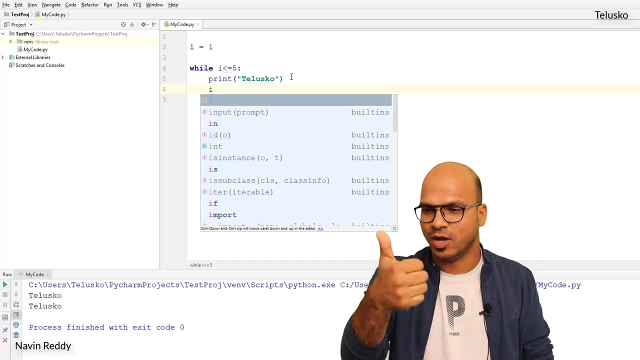 which is I in this case, and check if the value of I is less than five. and every time you print that is, go, just increment the value of I, right, So, because you're doing it right. So you're saying hello, hello, So you're incrementing the value, So you will say I is equal to I plus one, That's. 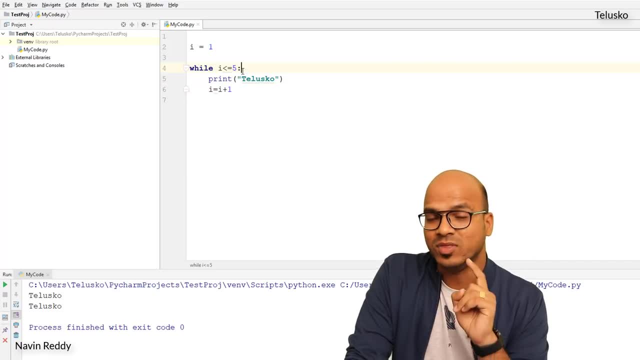 right, So you have to specify the condition and a colon. Now this colon specifier- whatever is coming ahead- is a part of this block And this two statement belongs to the same suit- is because we are using a proper indentation here And now. let me just run this code and you can see we got. 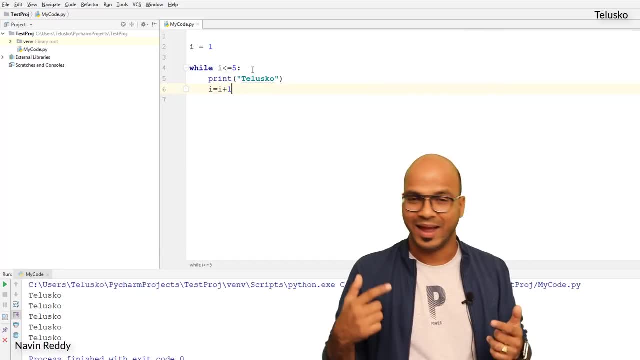 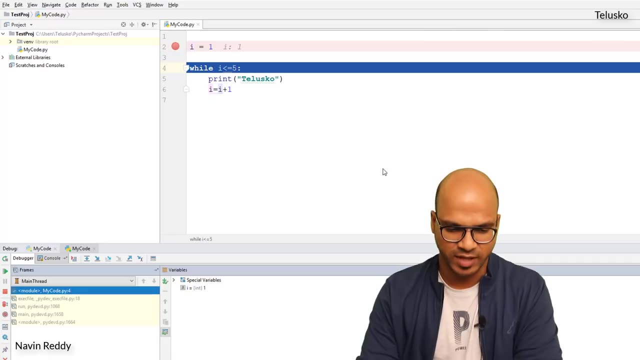 telescope five times. So what is happening behind the scene And how do I know that? It's very simple. So let's set the breakpoint and now let's debug it. I love this thing, debugging- And then say F8.. And you can see the value of I is one. Okay, that's done. 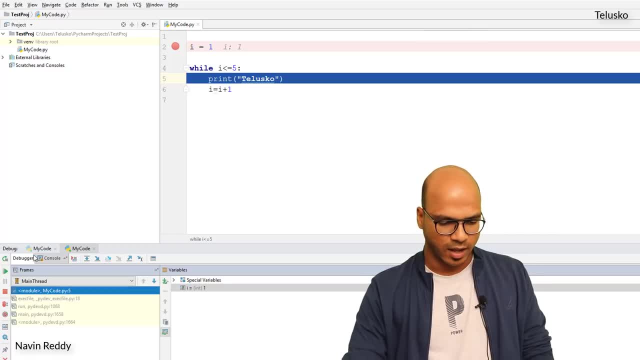 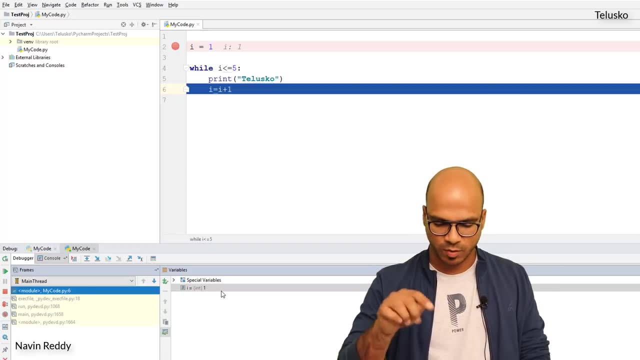 And then, if I can say F8, it is printing telescope once And you can see that in the console. Okay, you can see that we got hello once. And if I go back to debug again the value of I now, So the moment I say F8, the value of I becomes two. You can see the value of I is two now And it will. 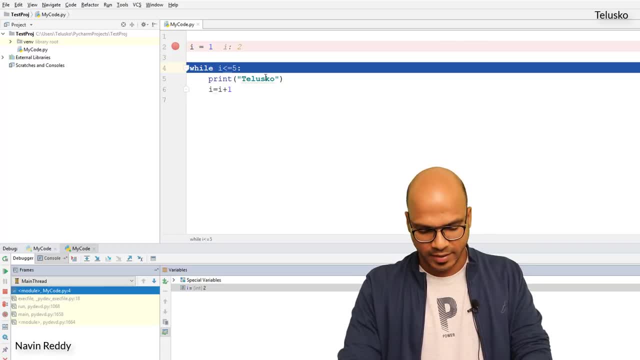 check. if two is less than five, Yes, it will go ahead and it will print telescope. You can see. if I go back to console, telescope will print second time. And then if I say F8 again, you can see we got value of: I is three, It's three, less than five. It's three less than five, It's three. 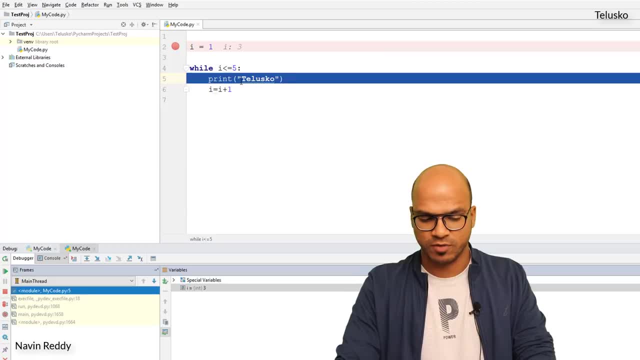 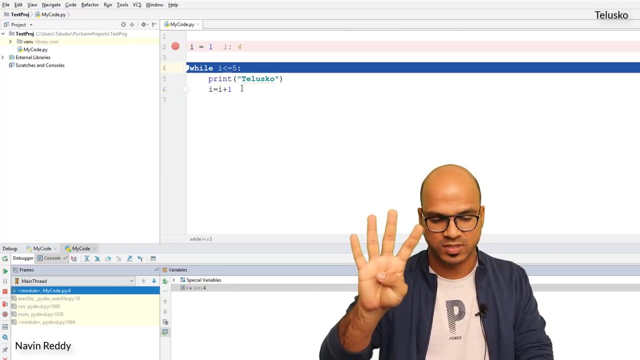 less than five. Yes, it will go ahead, it will print. It will then try to print the statement, which is: which is telescope? And you can see in the console we got telescope three times And now the value of I is four, Right, So if you can see the value of I is four And then if I say F8, it. 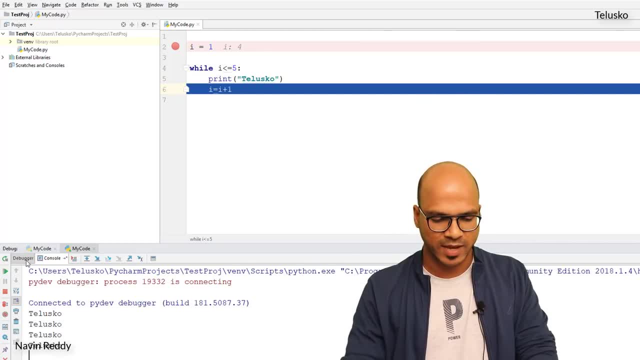 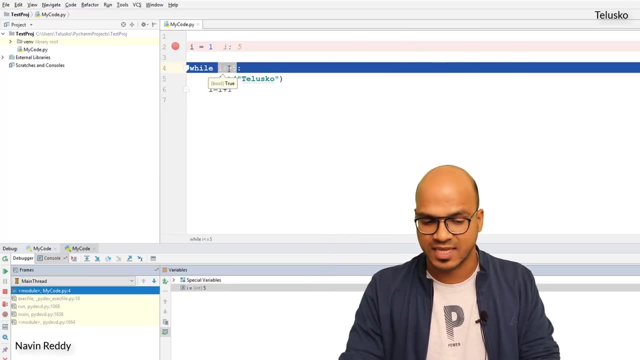 will print telescope fourth time. You can see that in console. If I switch back to there you can see we got telescope four times. And then the value of I now is five. Right, Is a five less than equal to five? Yes, you can see, we have equal to there. The evaluation is also true. You can see that the pop 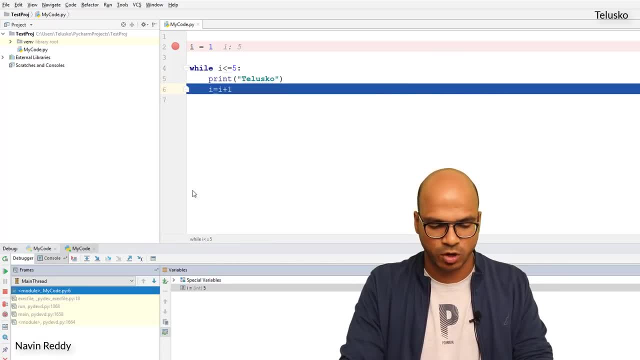 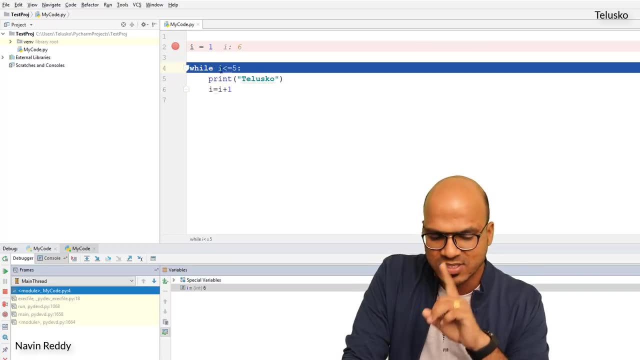 up is false. It will print telescope fifth time. You can see we got fifth time. And if I go to debugger again, say F8 and you can see the value of I is six. Now the value of I is six. Right Is six. 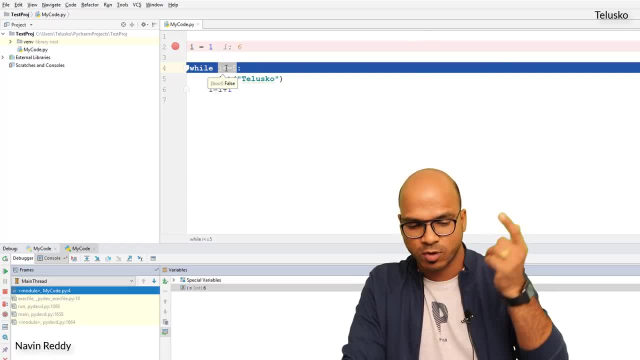 less than equal to five. No, that's a false Right. You can see the. you can see the pop up is false And if I say F8 now, it will come out And that's why you've got five times telescope Right. So 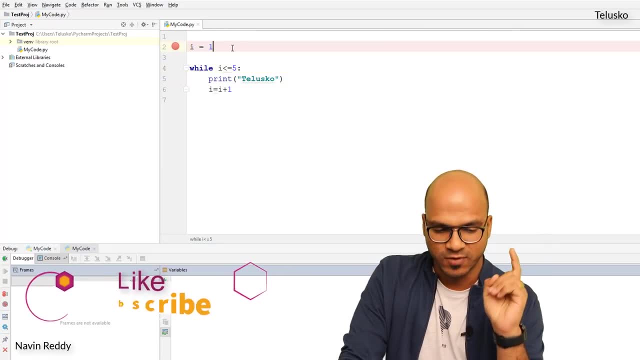 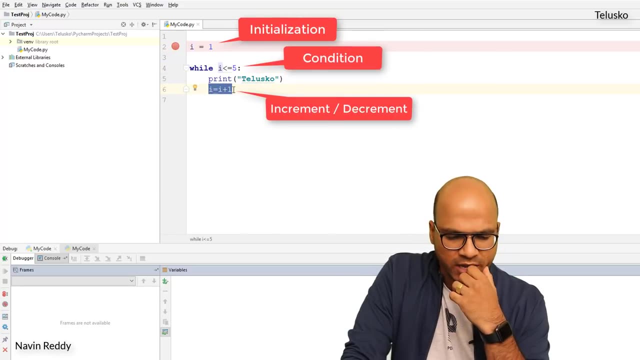 these are. you can use while loop. Now, three things are important here. First is the initialization, Second is the condition And third one is increment. Oh, can we do decrement here? Yes, we can do decrement as well, So you can do reverse. 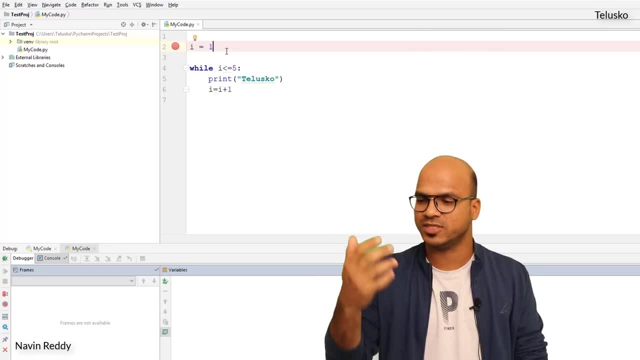 Right, Sometimes we go in this way: Hello, Hello, Hello, Hello, Hello. Or we can say: So, let's say, we will do reverse: Hello, Hello, Hello, Hello, Hello, Right, So we can do that as well. So we 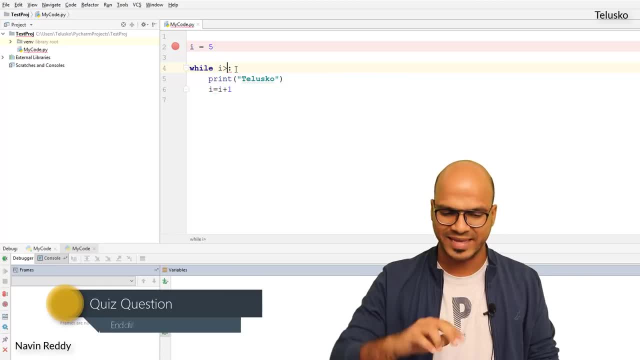 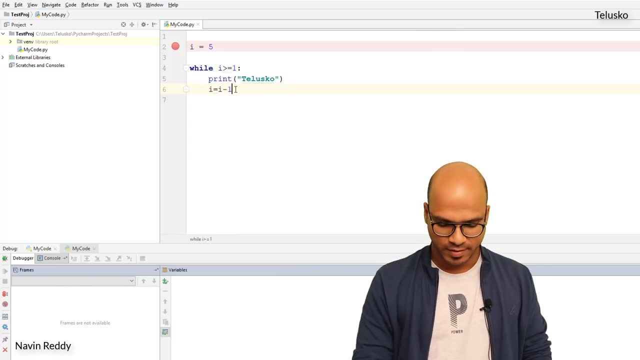 start with five And then we'll reverse the condition. We'll say I is better than equal to one, And instead of saying I is equal to I plus one, we'll say I is equal to I minus one. We are going in reverse order. Let's run this code. It works. You can see we've got five times hello. 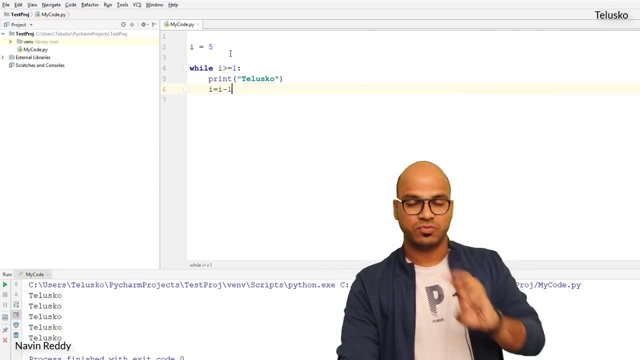 So we can go ascending, We can do descending, your choice. So there are three things important here: One, assign the value, then condition and then increment or decrement. Now let's say I don't want to print telescope here, I want to print the value itself. Or maybe I want to print telescope. 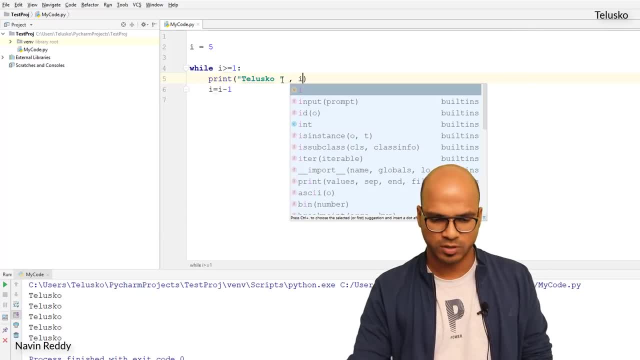 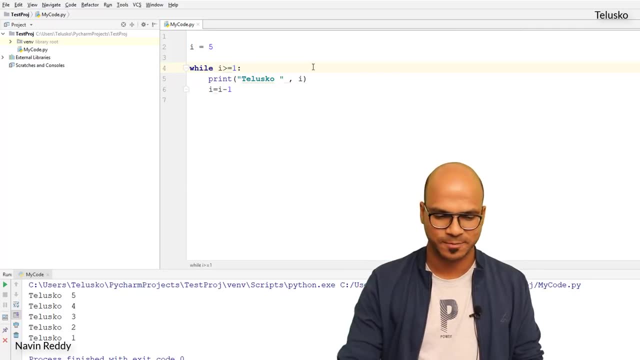 with the value. We can do that. So we can say: space comma: I. I want to print the value of I as well. Let's run this code and you can see it is printing. telescope five: telescope four: telescope three: telescope two: telescope one. So you can do that. OK, This is how you. 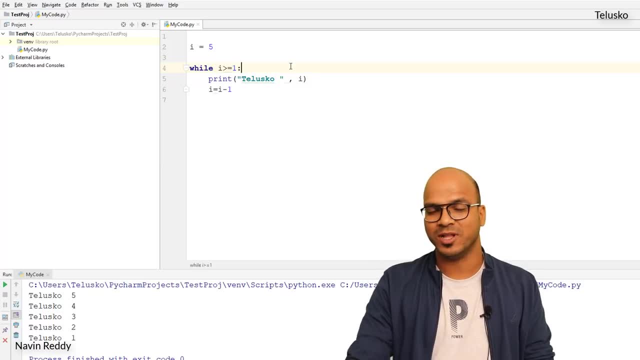 work with while loop. Now can I use multiple, like multiple vials, I mean while, inside of while. you can do that, So we have done that before as well. Right Example: I will print telescope once and then, while I'm printing telescope once, I want to print telescope rocks. 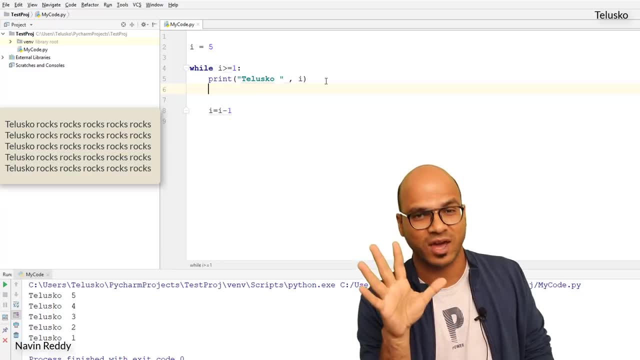 multiple times. I want to print telescope rocks. I want to print rocks five times. So what I'll do? I will say while: Oh, now I want to say five times, I have to use a different variable. right, And I will be using a variable here which is J is equal to one, again, We'll. 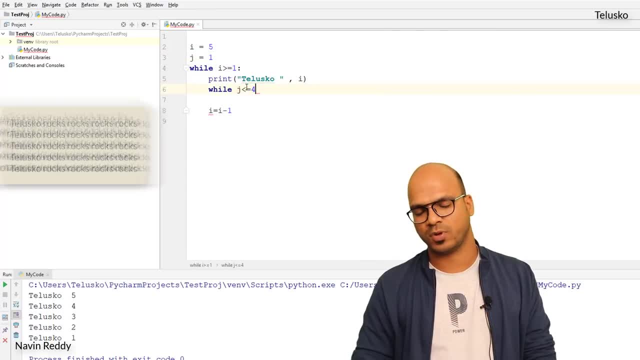 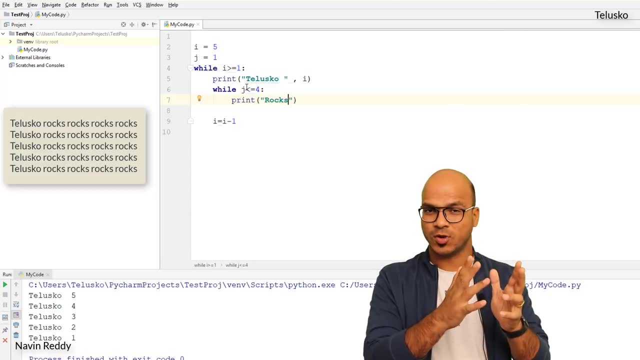 say J less than equal to four. Let's say I want to. I want to print rocks four times. We'll give a colon and we'll say: print rocks, That's good. So it will print telescope and then rocks four times. I don't. 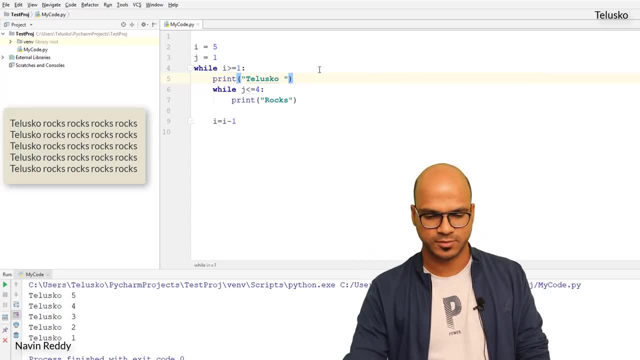 want to print the value of I now. So it will print telescope and rocks four times. So before executing this, you try to guess the output. OK, It's you, it's depend upon you. now You tell me what's the output. OK, Will it print telescope rocks four times? See telescope. 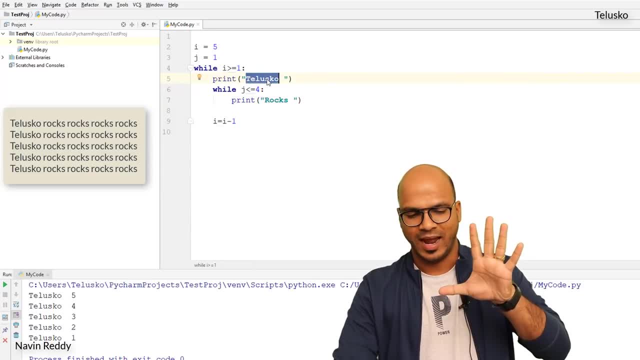 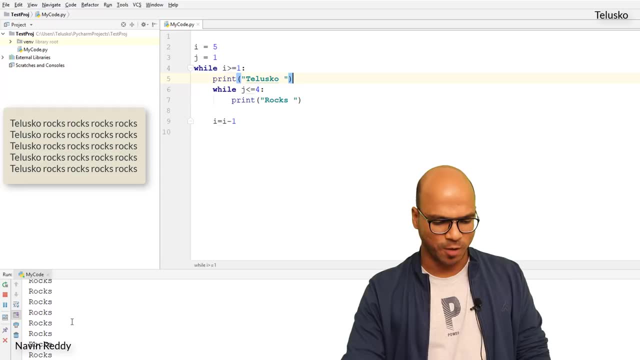 itself will get, will be getting printed five times Right, And then, on every line, you will get rocks four times. This is what you want, Right? But if I run this code- Oh, that's weird- It's not stopping anywhere. You know why it's not stopping? because we forgot to increment the value of J, You know? 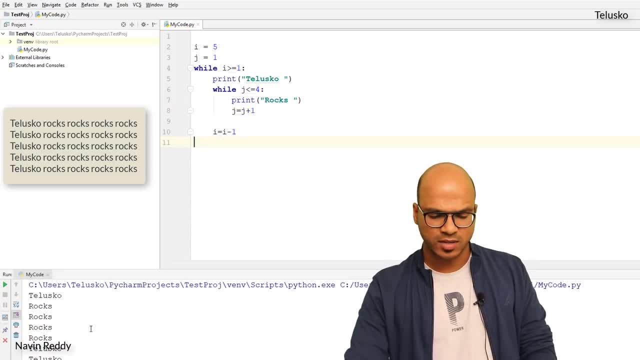 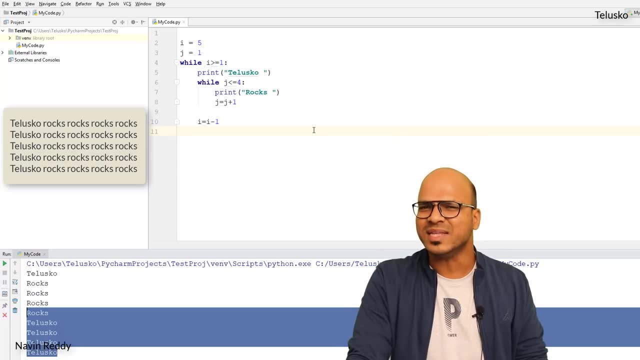 you learn from mistakes. Let's run this code once again And you can see we got telescope, rocks, rocks, rocks four times and then again telescope four times. That's that's. that is not something which we want. What is going wrong here? Let's try to debug this, you know. 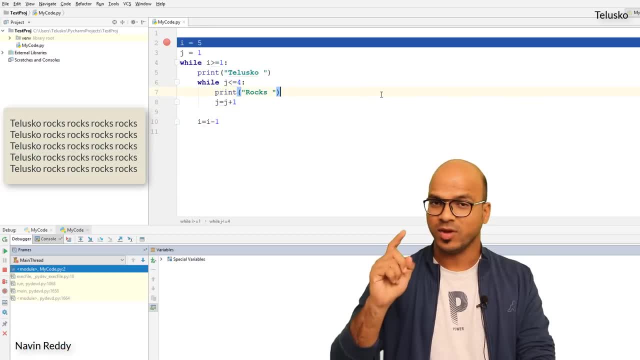 So I will just say, hey, debug the application. Now you can see, value of I is five, In fact. you know, just to make it more simple, Let's go with one, Let's go with increment, so that it will be easier for understanding. 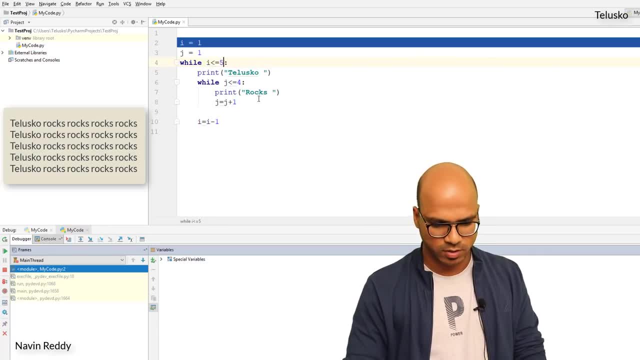 Because once you understand the basic stuff, you can try it on your own. I know this. we are using while inside a while. OK, So this is nested while loop. Let me just debug this by applying a breakpoint. Let me say F8, and you can see the value of. I is one, Remember. 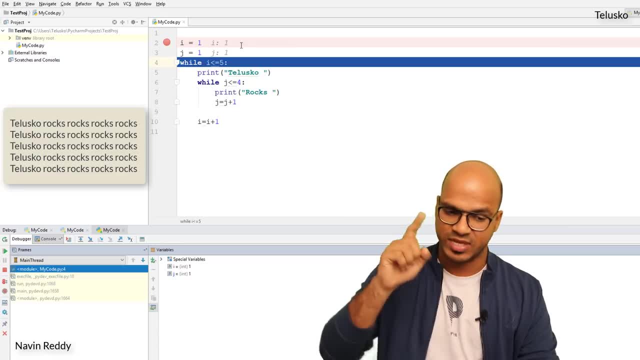 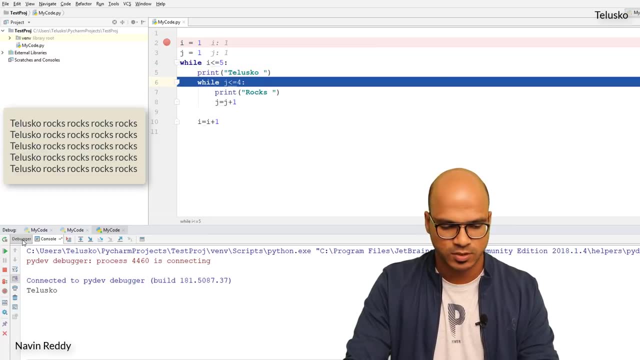 this values. The value of J is one. is one less than five? Yes, Let's go inside. It will print telescope, Of course, And you can see in the output console. we will be getting telescope now. We got telescope. Now, what's the value of J? It's one, One less than four? Yes, It. 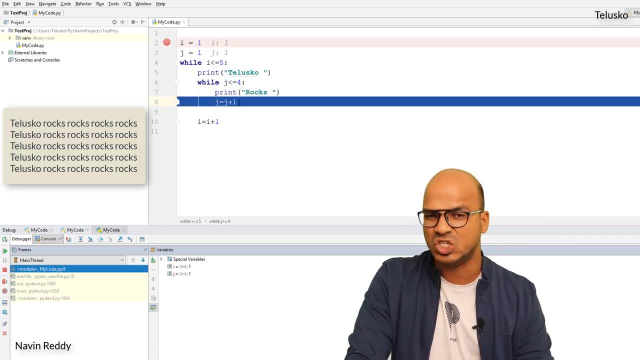 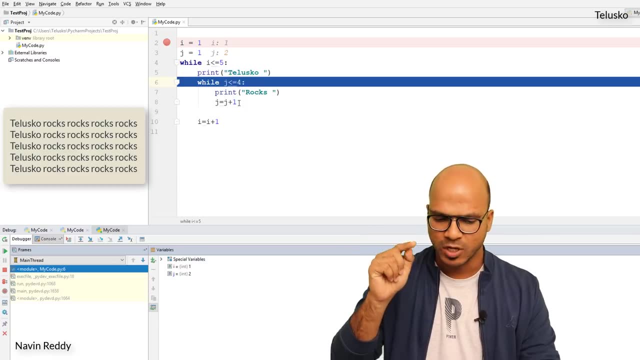 will go ahead, It will print logs, It will execute this: J equal to J plus one. So now the value for J is two. If I say F8, the value of J is two. But look at the jump. It is not jumping outside, It's not jumping back to this loop, It is jumping back to the inner. 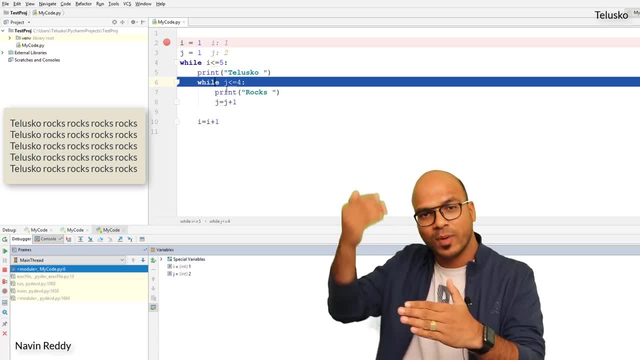 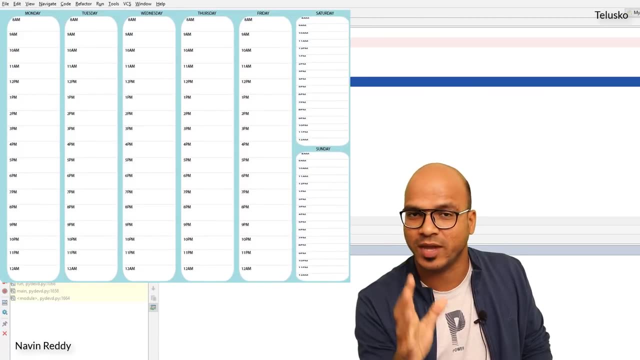 loop, because first it will complete the inner loop, then it will go back to the outer loop. Right, It is something like you know, we have seven days a week and each day has 24 hours. Right, The number of hours is the outer loop and the number of hours is the inner loop. Right, 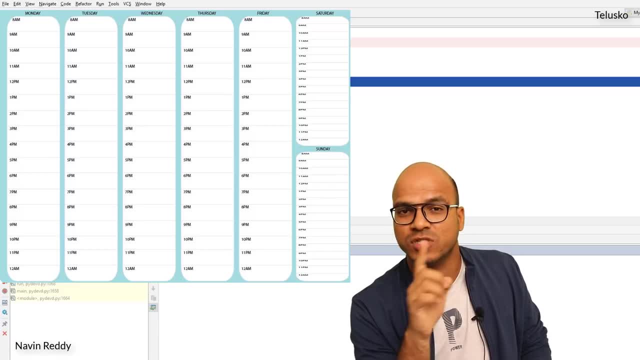 So what it means. So let's say, if you start with Sunday, Sunday has 24 hours. It will start with 0th hour, then 1 hour, 2nd hour, 3rd hour, 4th hour, Now when you complete. 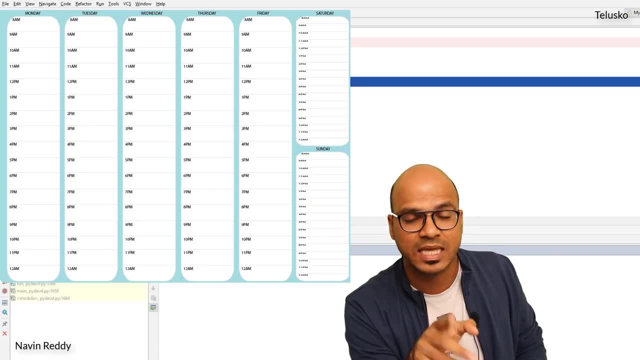 the entire 24 hours. it will go for the new day, which is Monday. in this case, On Monday as well, we have the same hours, Right: 0th hour, 1th hour. So that means every time you change your day it will restart the number of counting for your hours. So it will first. 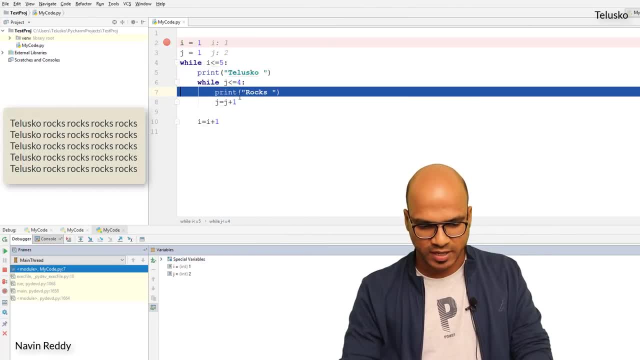 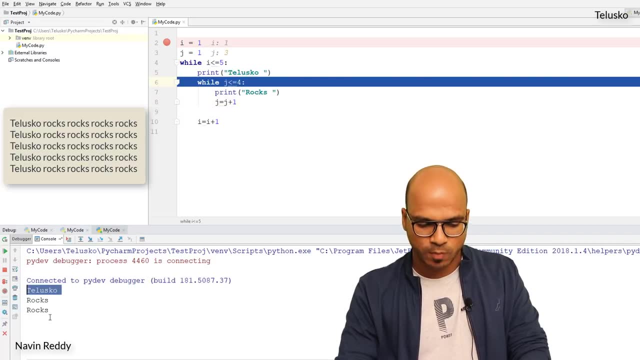 complete the hours Right. So the same thing is happening here. Let's say F8 again, It prints rocks. It will increment the value of j to 3. And that's why you can see, if you see the output, we got one thaliscope but two times rocks. Okay, 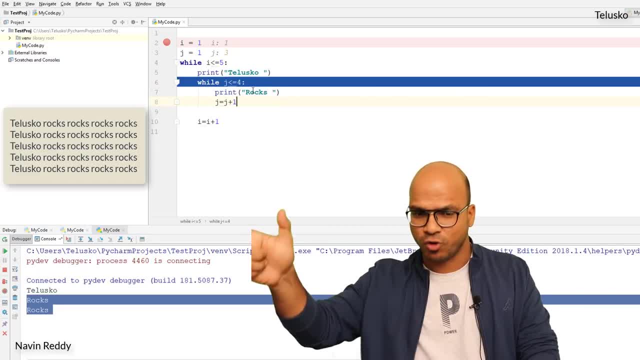 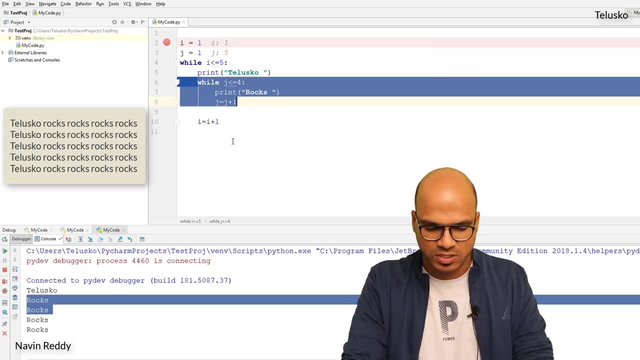 So that works. In fact, we wanted this Right. We wanted one thaliscope and four rocks. Okay, We'll do that. We'll think about that. If I run this, you can see we got rocks. and once it is getting completed, once the value of j it becomes 5, you can see that the value 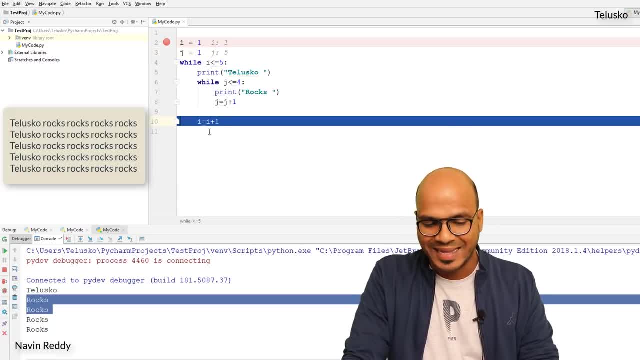 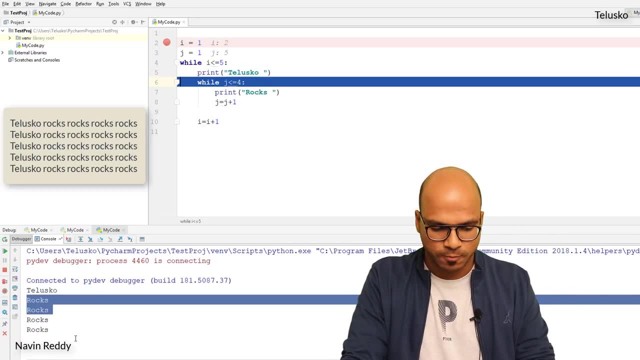 of j now is 5.. If I run this again, it is false and now it is focusing on i, So i value is 2 now, So i add there. and then again, if I say F8, it will print thaliscope, of course, But look. 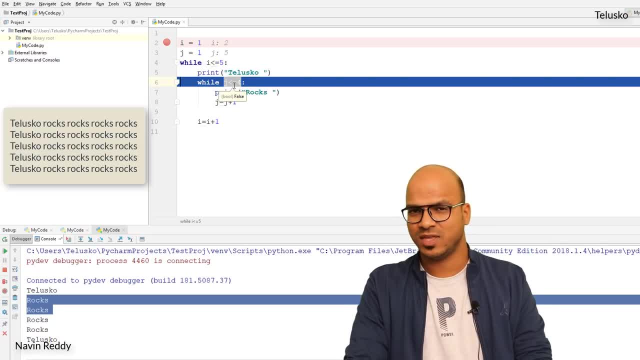 at the value for j. j is 5.. That's where things are going wrong. Now, since j is 5, it is not continuing ahead, So that was a mistake. So, to solve this problem, what we can do is first, we have to do two things. I want to print rocks on the same line, Right? I don't want. 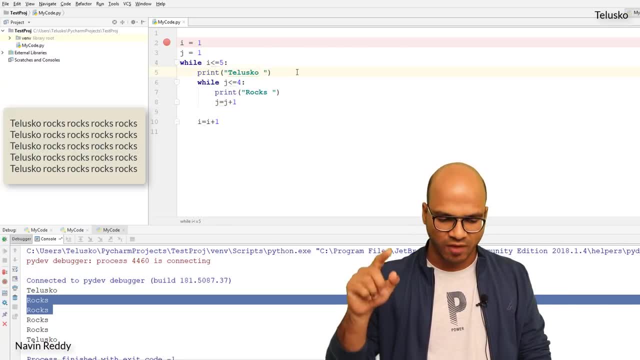 to print rocks on new line. So what we can do is: after thalisco, I can give a comma and say: end is equal to double quotes. Now what it means By default when you say print, it will print this statement and comes on new line. I don't. 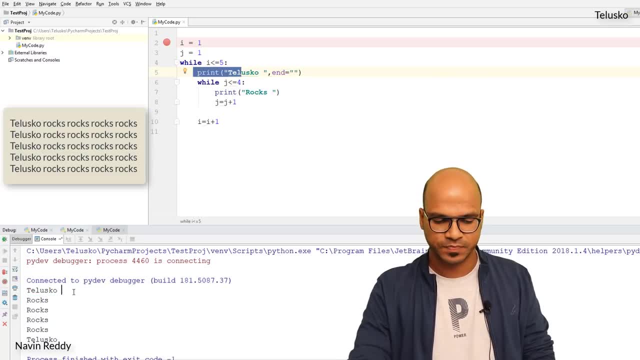 want new line. I want to print on same line. Example here: if you see it is printing thalisco and then it is coming on new line. I don't want that. I want it to be. I want it to print thalisco and stay on the same line. Same thing can be done for rocks. I would say, hey, don't. 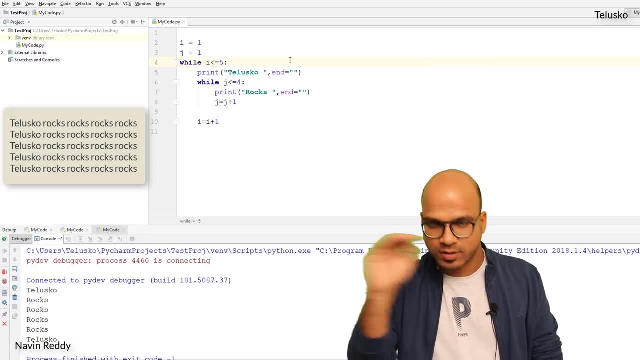 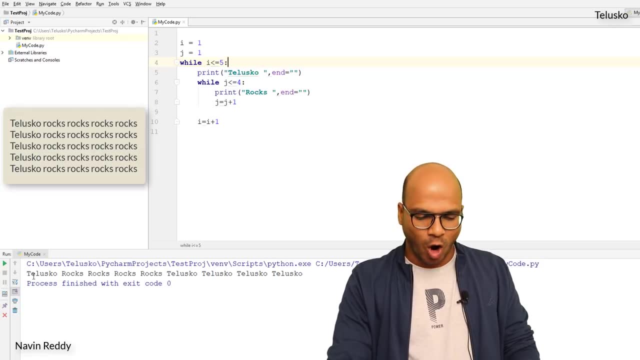 go on new line, stay on the same line. Now I hope it will come on same line If I say run Okay, So that we got everything on same line. Okay, We don't want that, We don't want. We want all thalisco on same line. We want thalisco on new line. So after incrementing: 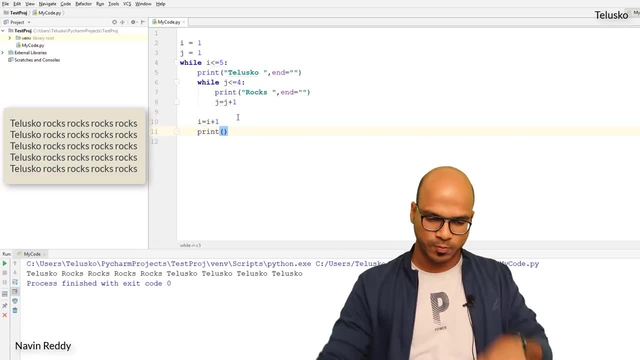 I will say print because, see, after completing one thalisco, I want to print on new line. So I will say run, You can see we got thalisco on new lines, but then rocks is coming only for four times here. What is going wrong? The value of j reached five here, Right. So 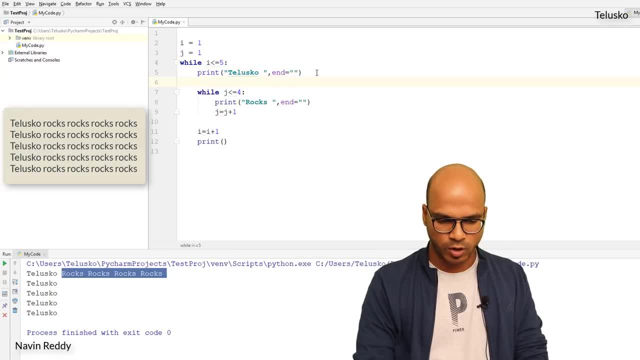 what I will do is, every time I start with the outer loop, I want to restart the value for j, which is one. It's important. every time, In fact, we don't. we should not be declaring the value here. Let's start here. Okay, So it will initialize here. Check for the condition. 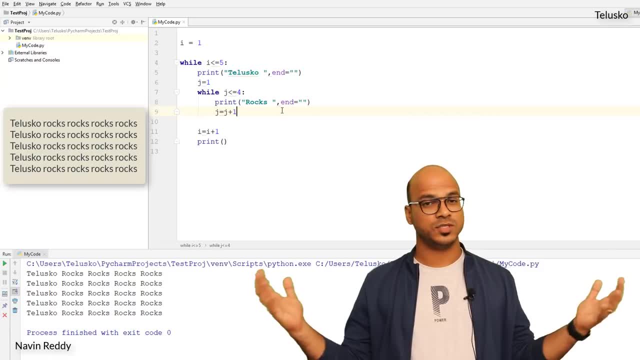 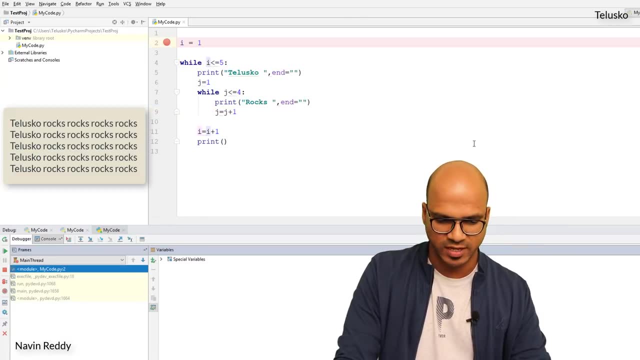 here and then increment, increment here itself. Let's run this. This we want, Right. So we got thalisco: rocks, rocks, rocks. Now how it is working. Let's again go for debug. We'll say debug and say f8.. You can see the value of: i is one, i less than five. Yes, it's one. 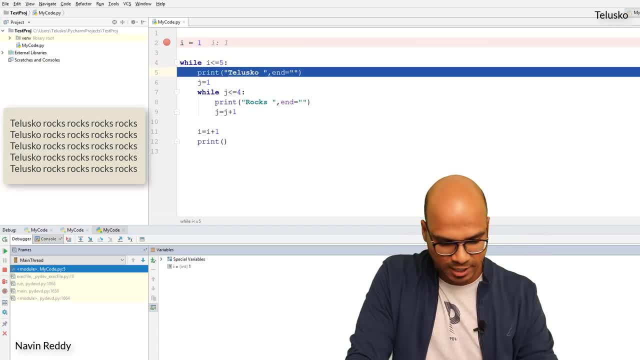 It will print thalisco and it will not go on new line. Okay, It will stay on the same line. Let me jump to console and you can see if I say f8, thalisco on same line. Okay, There's not jumping to next line. 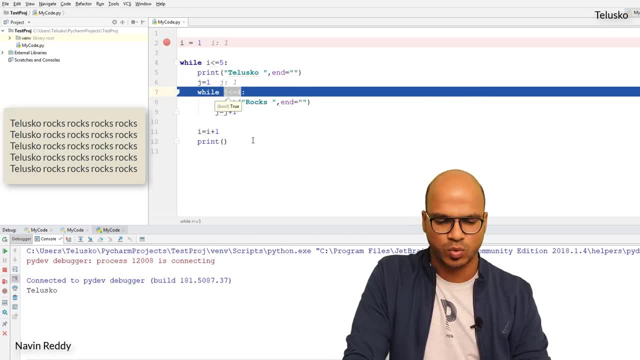 The value for j is one Is one less than four. Yes, It will go ahead and it will print rocks and you can see rocks on the same line and then the value of j is getting incremented to now, So you can see the value for j is two here, and then again it will come back. 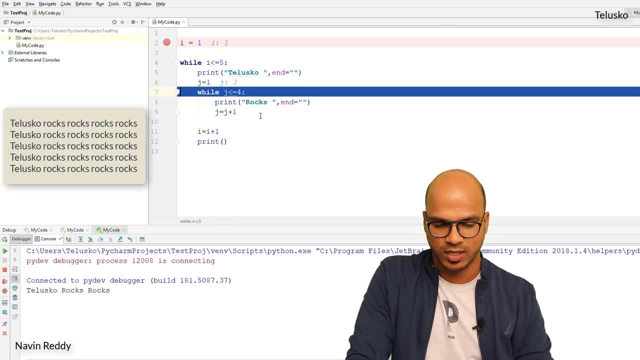 It will print rocks and it will go for j value, which is three, and then it will again: three is less than four. It will print rocks and then j value is four and then it will check: is four equal to four? Yes, it will print rocks and the value for j is now five. 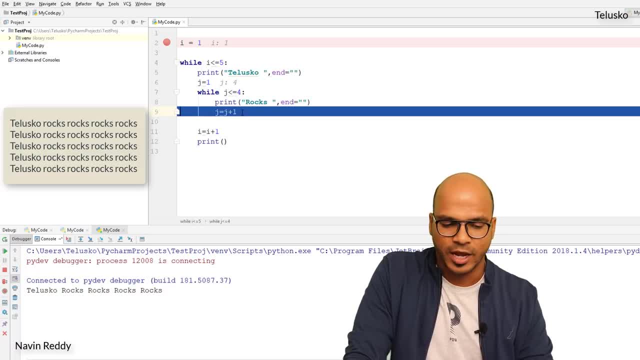 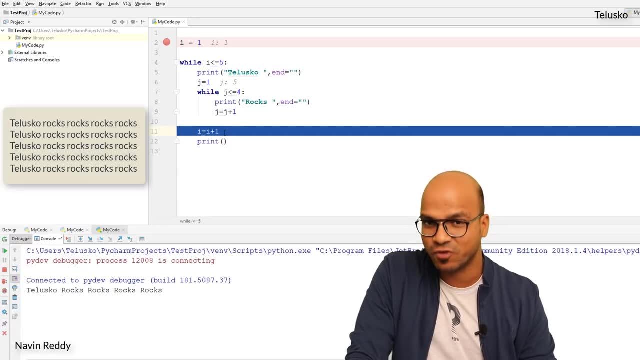 Now, five is not less than equal to four. It will come out, But where It will come out, to this next item, which is: i is equal to i plus one. Now, in this case, i equal to i plus one, It will increment the value for i, So it will make it two. and then, since we are, 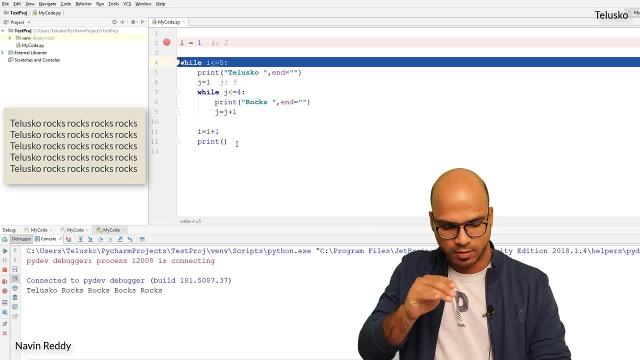 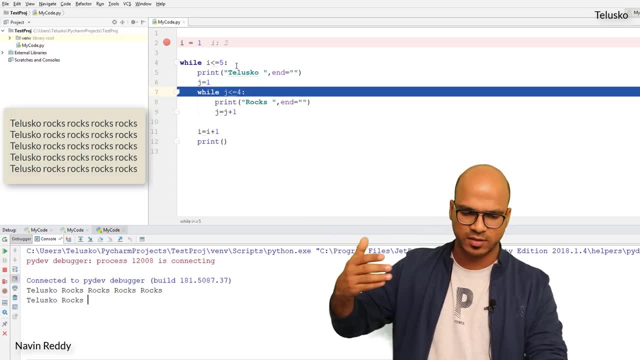 printing. if we, since we are doing print, it will come on new line. You can see the cursor. now Cursor is on new line. I will say, I mean it will continue. Okay, So it will do the same thing which we have done till now. So if I go fast, fast, fast, see that, See the sequence. 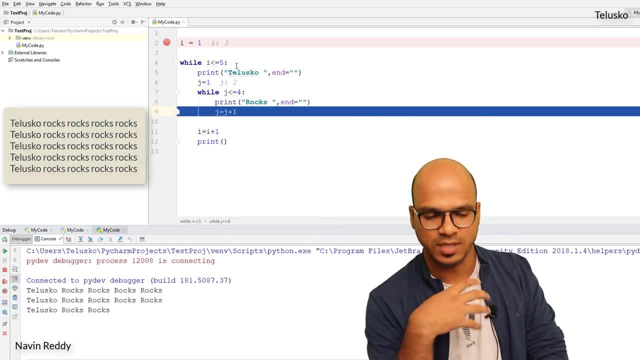 So this is how your- your loops are working Now if I go fast, fast, fast. see that, See the sequence. So this is how your- your loops are working Now if I go fast, fast, fast. see that. See the sequence. Now see, since I am doing this, I have worked on this for a long time.